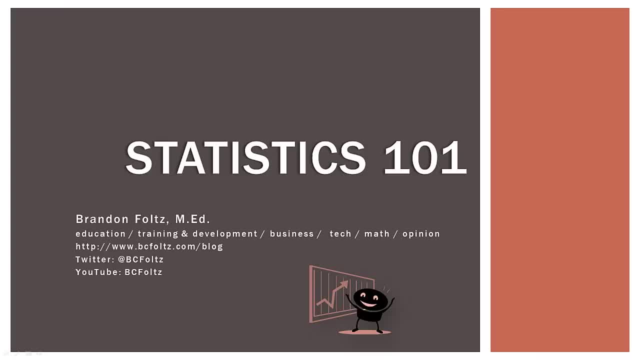 If you're watching this, it means you've accomplished quite a bit already. You're very smart and talented, but you may have just hit a temporary rough patch. Now I know, with the right amount of hard work, practice and patience, you can work through it. 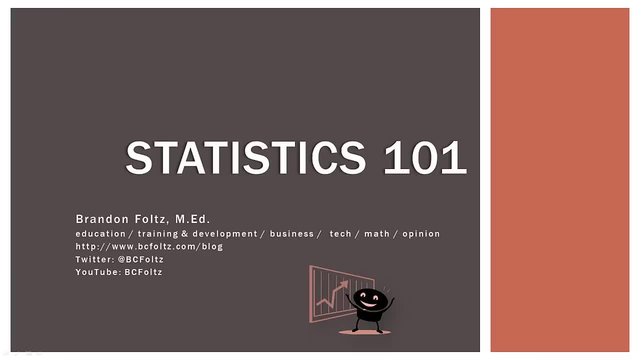 I have faith in you. Many other people around you have faith in you, So so should you. Number two: please feel free to follow me here on YouTube, on Twitter, on Google+ or on LinkedIn. That way, when I upload a new video, you know about it. 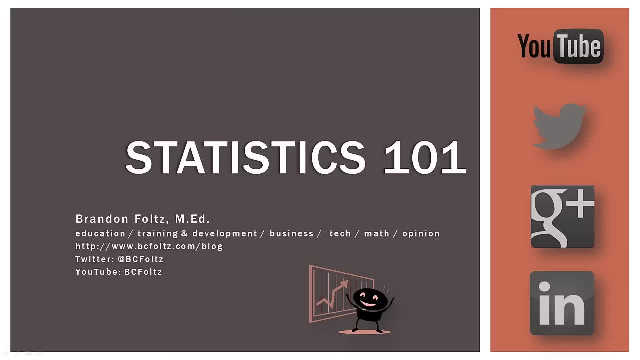 And it's always nice to connect with my viewers online. I feel that life is much too short and the world is much too large for us to miss the chance to connect when we can. Number three: if you liked the video, please give it a thumbs up. 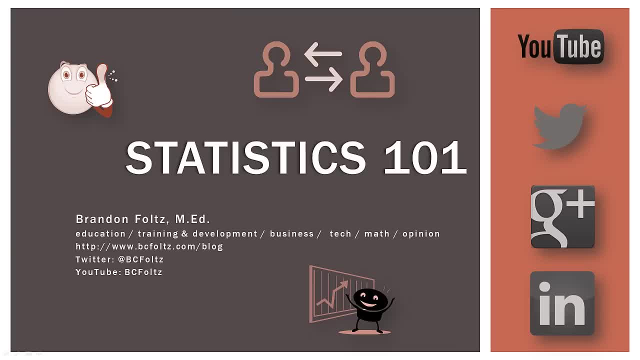 Share it with classmates or colleagues or put it on a playlist. That does encourage me to keep making them for you. On the flip side, if you think there's something I can do better, please leave a constructive comment below the video and I will take those ideas into account when I make new ones. 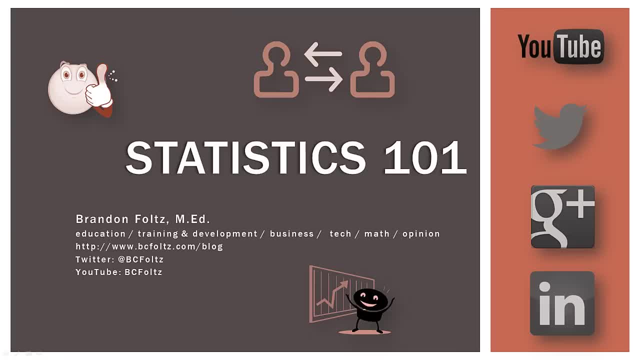 And finally, just keep in mind that these videos are meant for individuals who are relatively new to stats. So I'm just going over basic concepts, And I will be doing so in a slow, deliberate manner. Not only do I want you to know what is going on. 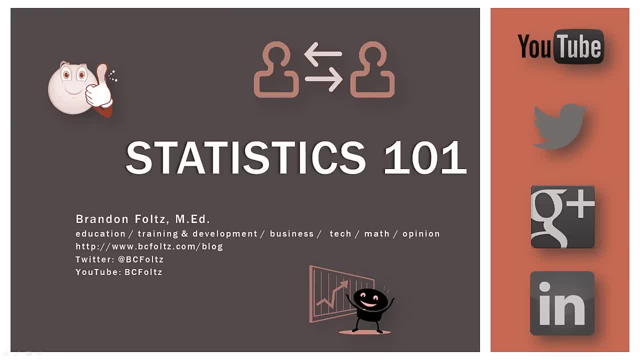 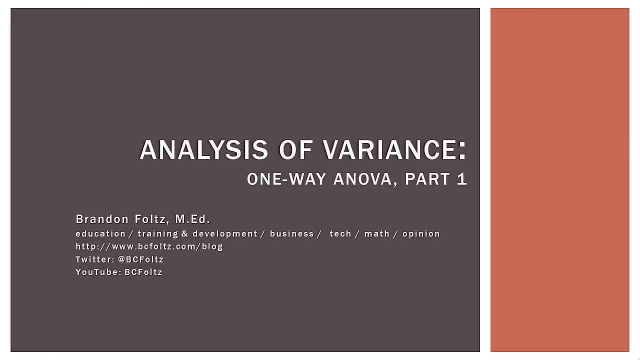 but also why and how to apply it. So, all that being said, let's go ahead and get started. So this is the next video in our series about the analysis of variance, or ANOVA. To make the topic more manageable, I've divided this video into two parts. 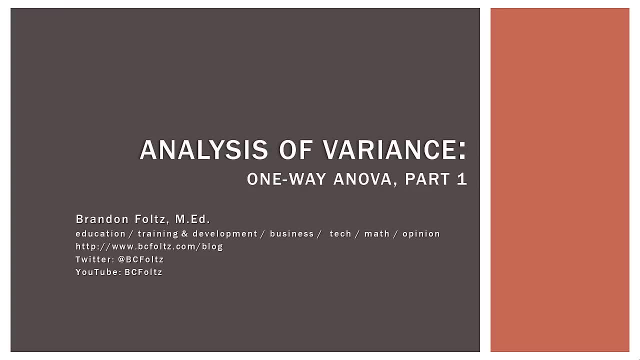 In part one we will discuss the conceptual background using graphics and charts and an example problem, And then in part two we will actually go into Microsoft Excel to conduct a hand calculation of ANOVA and also solve our example using Excel's built-in data analysis tools. 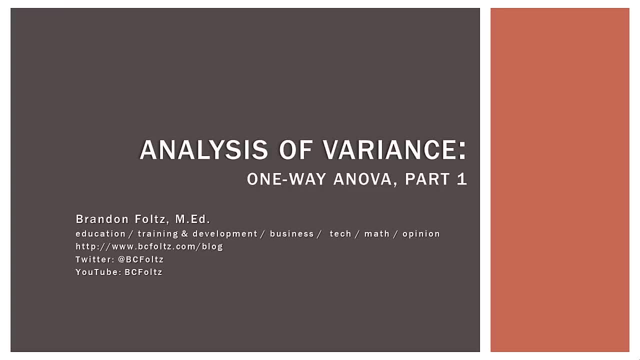 If you're watching this video on YouTube, you can download the Excel file using the link in the description, so you can follow along when we get to part two Now. in our last video, we took an in-depth look at the conceptual foundations. 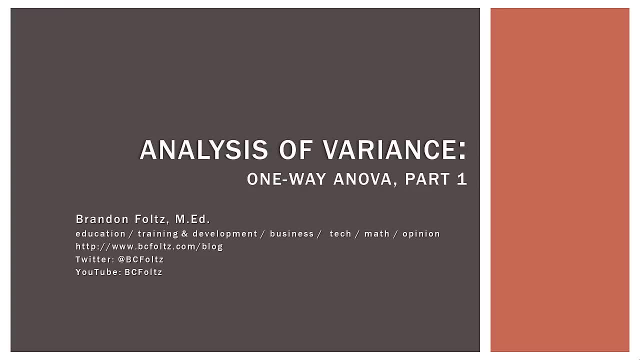 of ANOVA and what it offers us. Prior to ANOVA, we were limited to conducting hypothesis tests about a maximum of two populations. ANOVA frees us of that limitation, permitting comparisons of multiple populations and even subgroups, or what are called blocks of those populations. 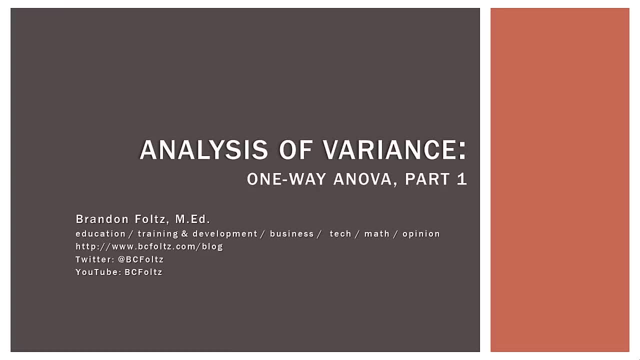 Now there are several types of ANOVA. In this video we will be focusing on what is called the one-way ANOVA, And in a later video we will discuss the two-way ANOVA. It is important to note that one-way ANOVAs go by other names. 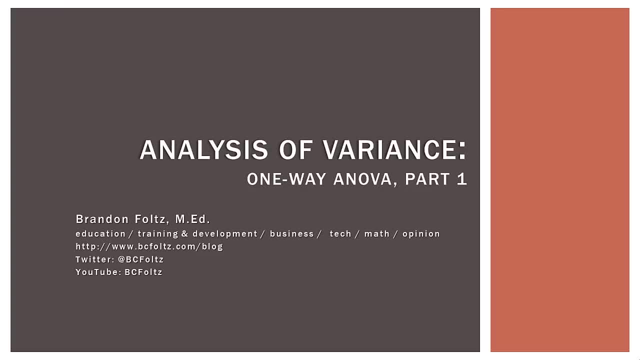 such as the single-factor ANOVA and, in experimental contexts, the completely randomized design. These are all basically the same thing, But this video is very comprehensive. In part one, I will use several illustrations to make concrete the abstract concepts underlying ANOVA. 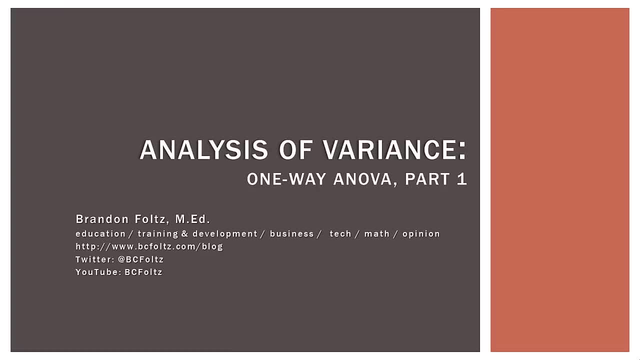 In part two we will go into Microsoft Excel to hand-calculate the ANOVA, which, admittedly, you may never actually have to do So. this video offers a solid, comprehensive conceptual foundation of one-way ANOVA using an example. problem with illustrations and graphics. 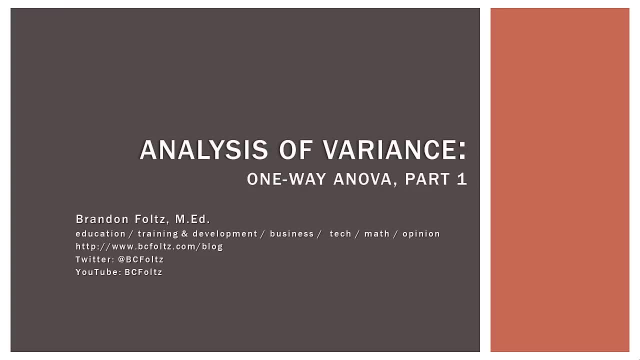 So, if you are new to ANOVA or are still trying to figure out exactly what it is, this video is for you. So sit back and enjoy. Sit back, relax and let's go ahead and get to work. 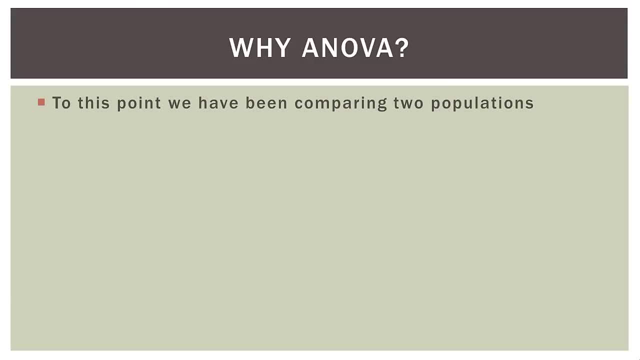 So the most obvious question is: why do we have ANOVA in the first place? So, like I said before, to this point we have been comparing two populations only, So we use the independent samples t-test or the matched sample or the paired t-test. 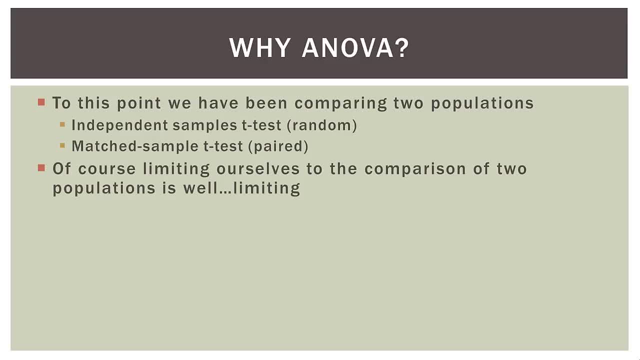 Of course, limiting ourselves to the comparison of two populations as well limiting. What if we wish to compare the means of more than two Populations? What if we wish to compare populations each containing several levels or subgroups? Well, that's why we have ANOVA. 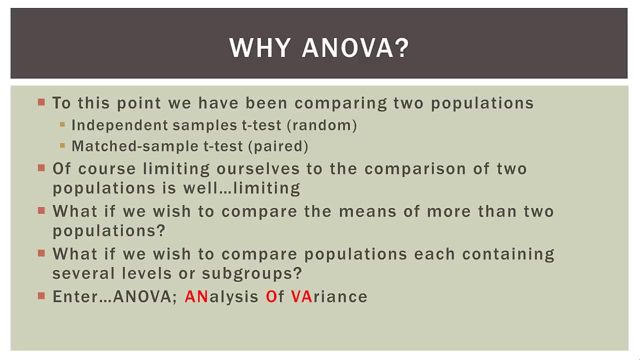 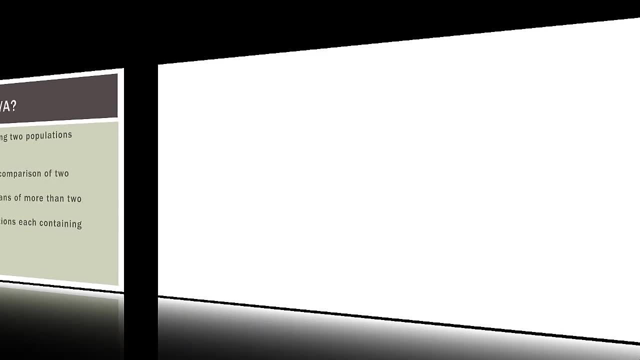 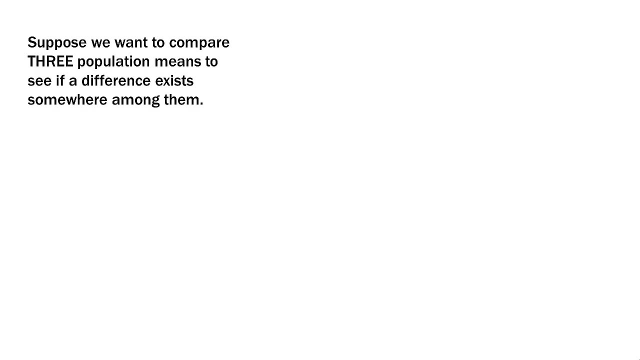 It allows us to do those things. And remember, ANOVA is an acronym that comes from the phrase analysis of variance. So suppose we want to compare three population means, like we will in this example problem, to see if a difference exists somewhere among them. 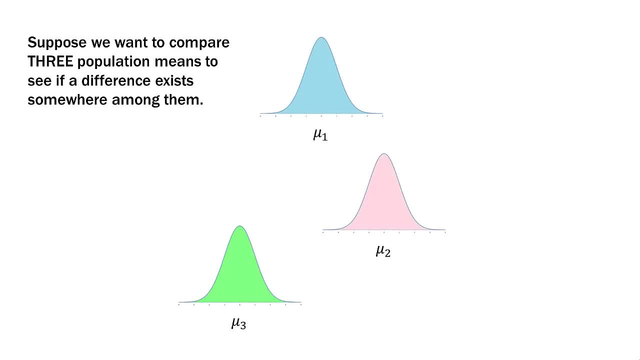 So we have population one here in the blue, population two here in the pink and population three here in the green, And each population has its own population mean. So mu one, mu two and mu three. So what we're asking is: do all three of these means come from a larger common population, sort of in the background? 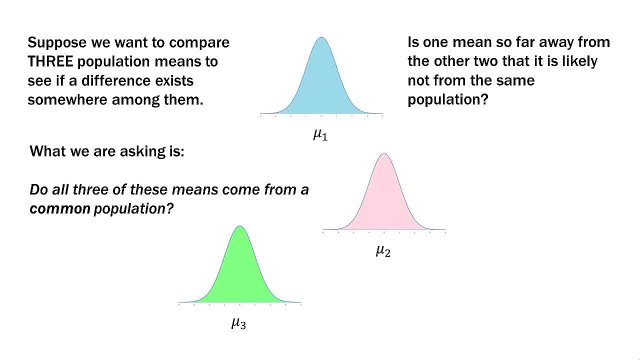 Or is one of the means so far away from the other two that it is likely not from the same population? Or are all three so far apart that they all likely come from unique populations? So really it's about distinction. Are all three of these populations common to a larger population, or is one or all three of them different from one another? 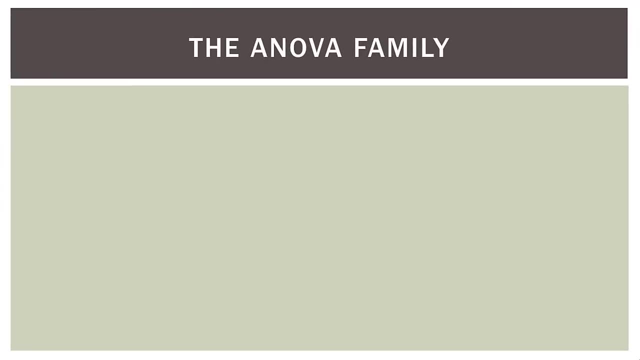 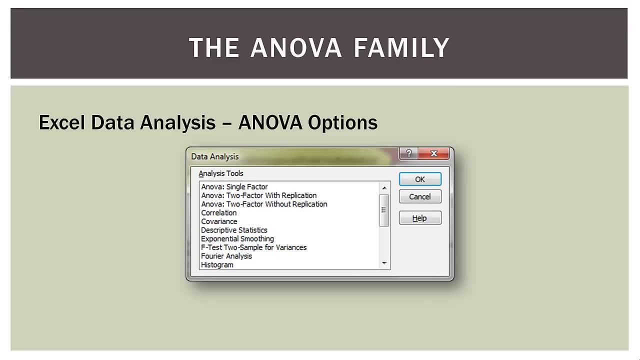 Now, I mentioned before there are several types of ANOVAs. So if you go into the data analysis section in Excel, you will see all those. So you will see ANOVA single factor, ANOVA two factor with replication and ANOVA two factor without replication. 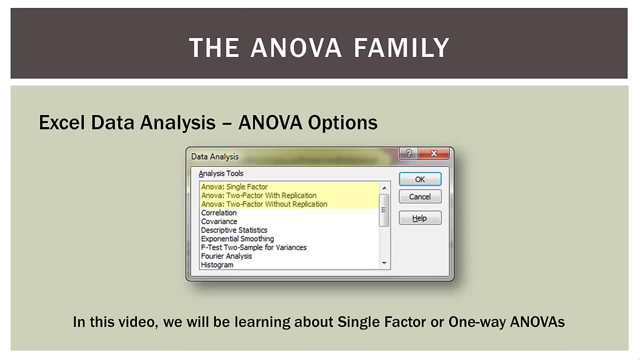 Now we will get to all those eventually, But for now we're going to be dealing with the first type. So in this video we will be learning about single factor, or single factor, Or one-way ANOVAs. 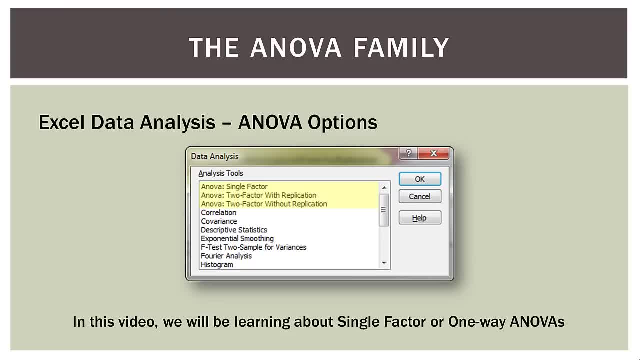 They are the same thing. So if you go into Excel and see this menu in the data analysis tool, I want you to know exactly which one we're doing. We are doing the ANOVA single factor or the one-way ANOVA. 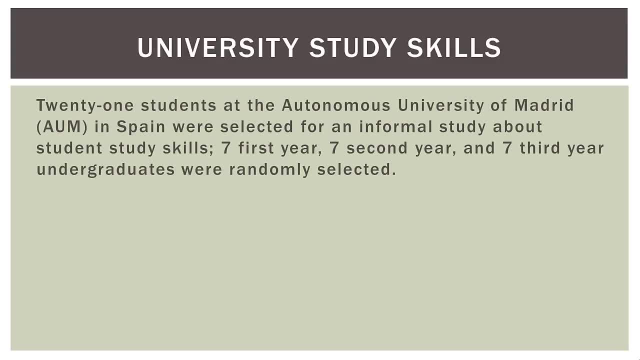 So here is our fictitious problem. So 21 students at the Autonomous University of Madrid, the AUM, in Spain, were selected for an informal study about student study skills. So seven first-year, seven second-year and seven third-year undergraduate students were randomly selected. 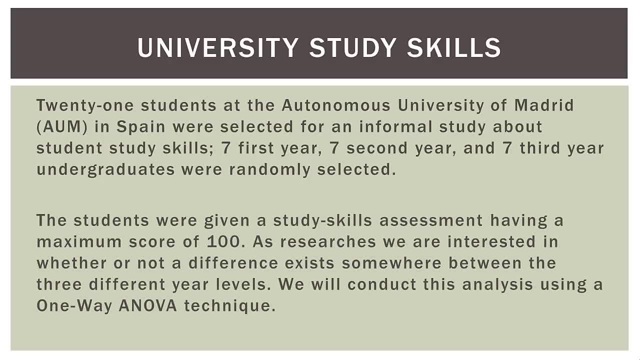 The students were given a study skills assessment, having a maximum score of 100.. Now, as researchers, we are interested in whether or not a difference exists somewhere between the three different year levels, So we will conduct this analysis Using a one-way ANOVA technique. 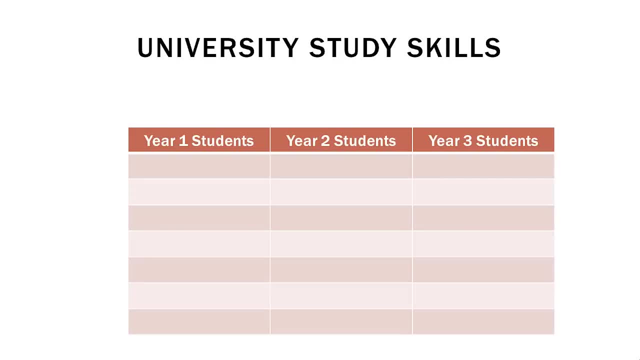 So here is our basic chart. So you can see that we have a column for each year of students. So these are our columns. Sometimes they are called groups And I mentioned in the previous video one of the challenges of teaching and learning: ANOVAs. 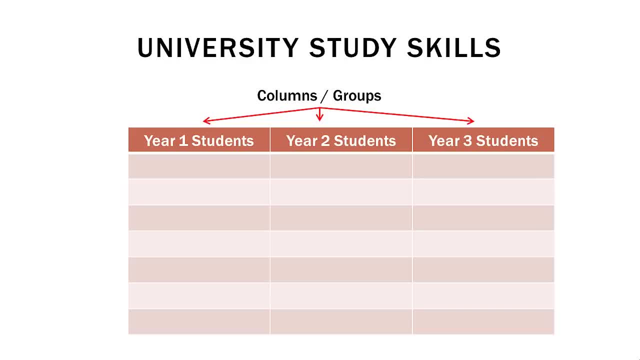 is that different professors and different textbooks will call the same thing different things. So sometimes these are called columns, sometimes these are called groups. Now, why is this called a single factor, ANOVA? Well, if you look at this chart, this year of student is a single factor with sort of several levels to it. 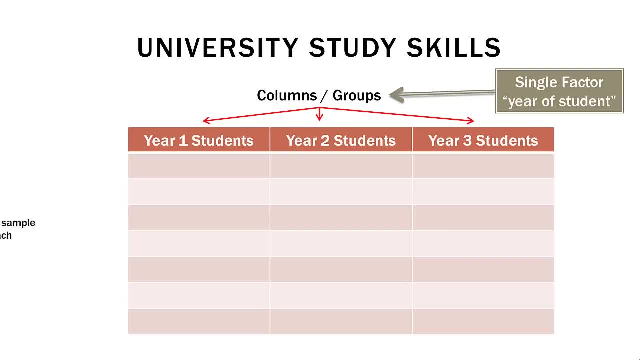 So that's why it's called a single factor. Now, within each year of student, we're going to select a random sample, In this case seven students. So if you get the geometry of the chart, you can kind of understand how it's all put together. 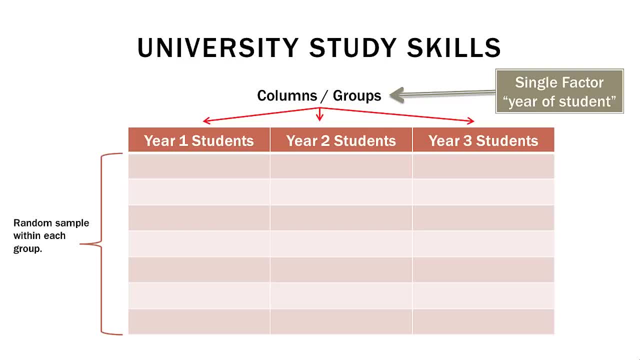 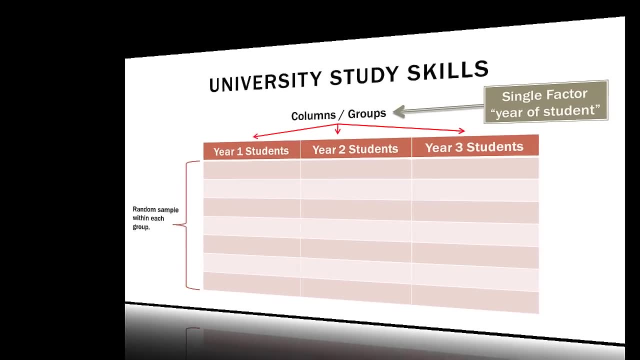 So we have three columns or groups. The single factor we're looking at is the year of the student And within each group we're going to be taking a random sample. So here is our actual data. So remember, these scores are out of 100. 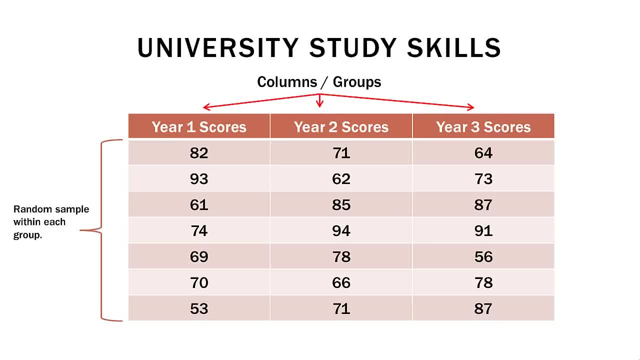 So you can see the seven year one student scores in the left, The seven year two student scores in the middle And the year three student scores over here on the right. Now remember that these are random samples within each year or each column, each group. 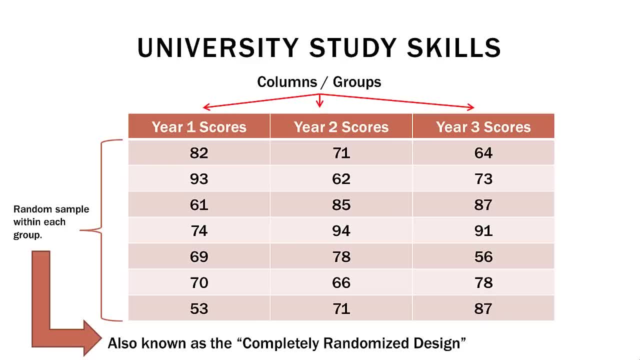 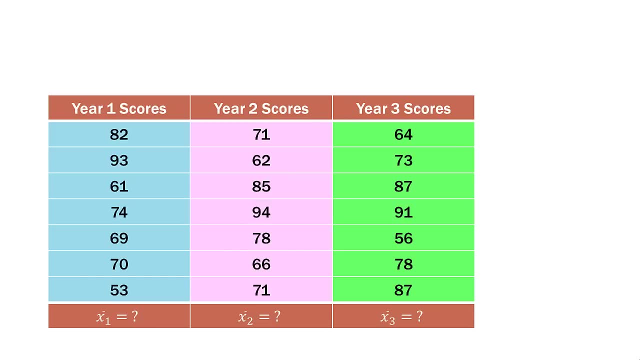 That's why, in an experimental context, this is called the completely randomized design. So you may see that in your class or in your textbook, or of course, both. So I went ahead and color coded each year so we can keep them distinct. 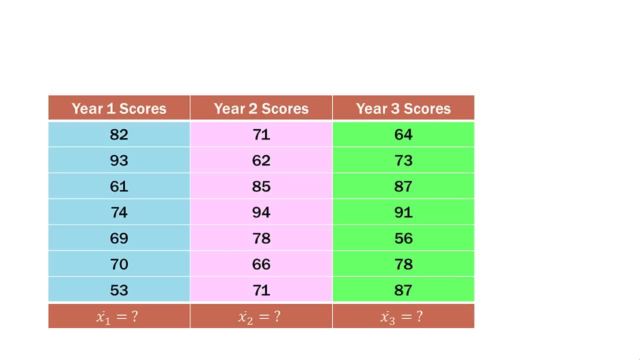 Now, if you notice, at the bottom here I have x bar sub one, x bar sub two and x bar sub three. Well, of course, that's going to be the mean for each column or each group, So each year will have its own characteristics. 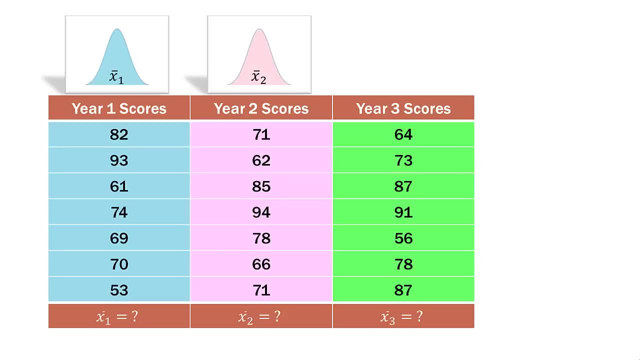 It will have its own mean and its own distribution or its own variance. So I went ahead and color coded those to match. Now there will also be an overall mean, Which is the mean of all 21 scores taken together. Sometimes this is called the grand mean. 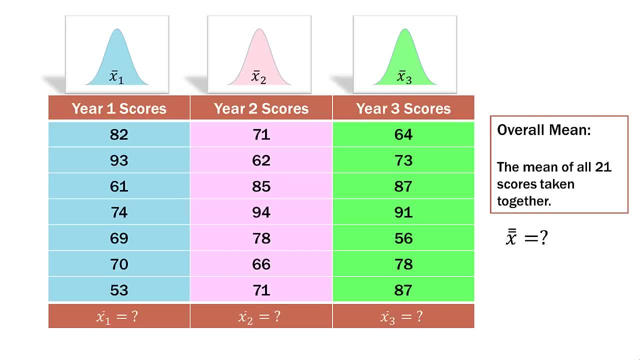 I call it the overall mean Same thing. So there are several means under consideration here. We have the mean for each column or each factor at level. It's the same thing, because our single factor is the year of the student. So we have x bar sub one, x bar sub two and x bar sub three. 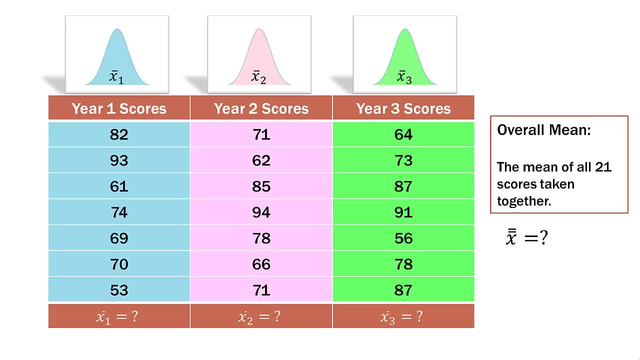 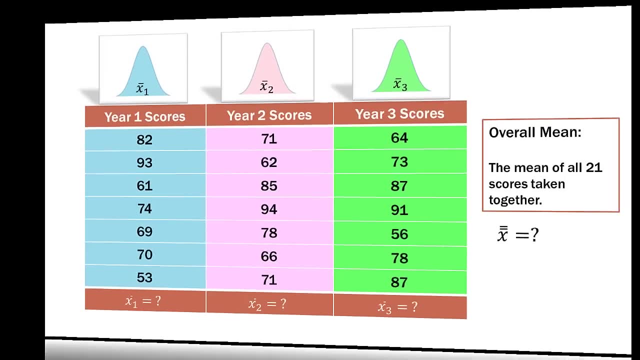 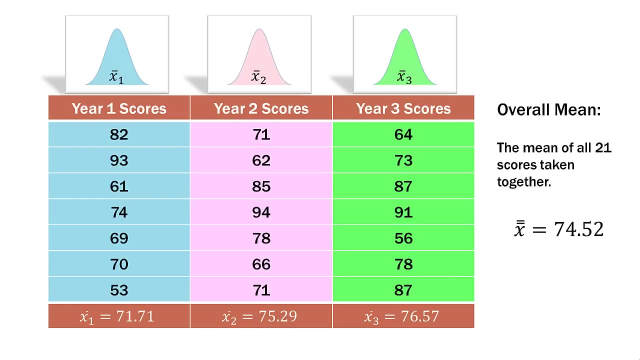 Then, of course, we have the overall mean, Or sometimes it's called the grand mean, Which is the mean of all 21 scores taken together. So the first thing we want to do is find the mean for each column and the overall mean over here on the right. 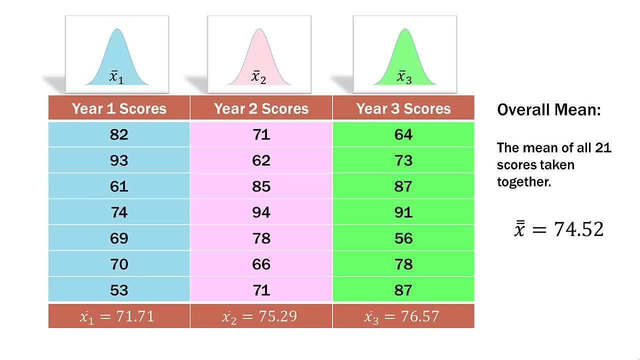 So the mean of the year one scores was 71.71.. That's x bar sub one. The mean of the year two scores was 75.29.. That's x bar sub two, Then x bar sub three, which is the mean of the year three scores was 76.57. 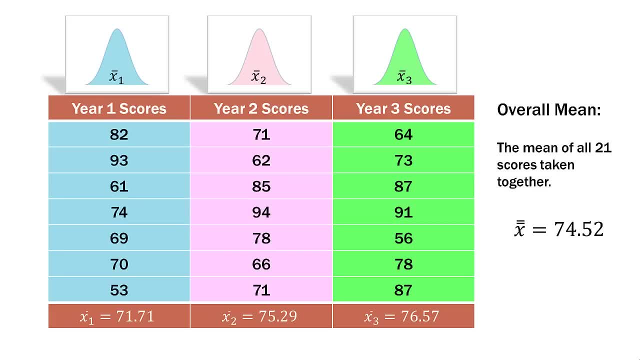 Now the overall mean, or the grand mean of all 21 of those scores taken together, is 74.52.. So that's the first thing we want to do when doing our hand calculation for the one-way ANOVA. So you can see our column means here on the bottom. 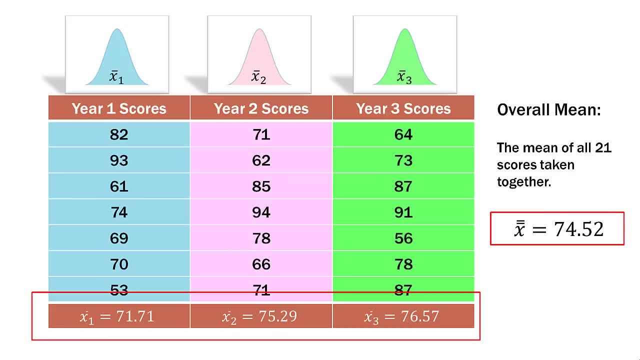 And our overall mean here on the right. Now, if we take a quick look at the column, means, what do we see? Well, we can see that the 71.71 over here for the year one students seems a bit odd. It seems a bit different than the other two. 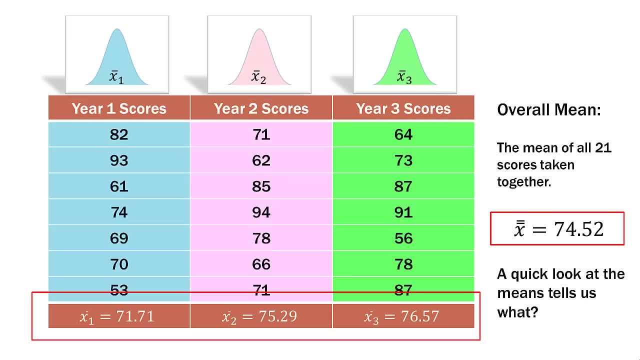 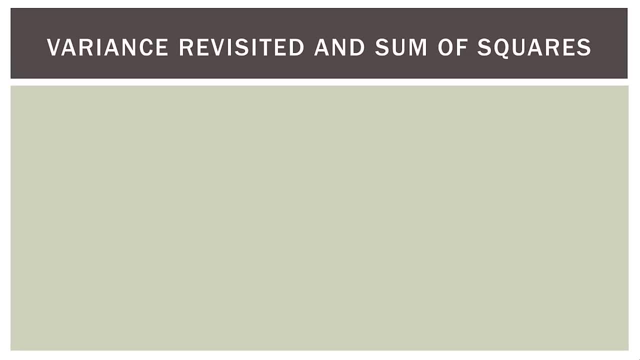 Now we don't know if that's going to be just due to natural variation Or there's actually something there. That's why we're doing the actual ANOVA. So let's briefly go back and visit the idea of variance and its related concept, the sum of squares. 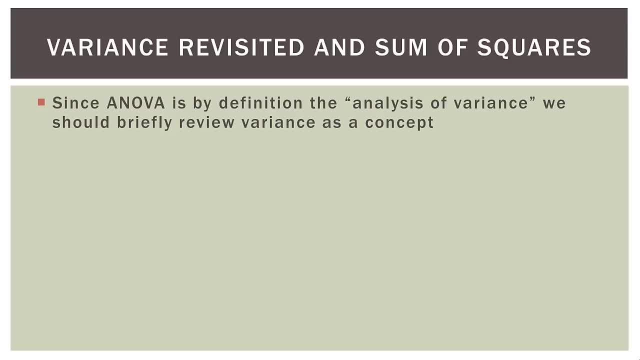 So, since ANOVA is, by definition, the analysis of variance, we should briefly review this as a concept. Remember that variance is the average squared deviation or the average squared difference, same thing of a data point from the distribution mean. So we take the distance of each data point from the distribution mean. 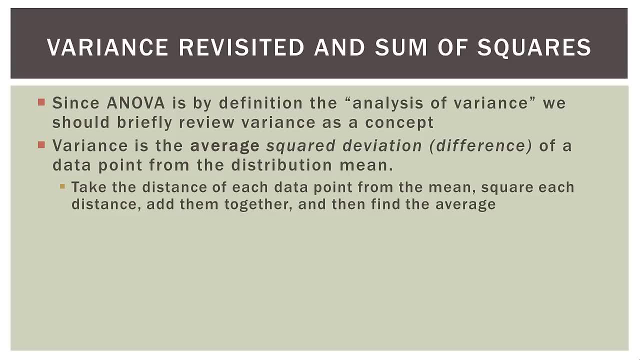 Square that distance, add those together and then find the average. That is variance. But if we take out that last step, if we take out the find the averages part, we are left with just the sum of the squares. So we would take the distance of each data point from the mean, square each distance and then add them together. 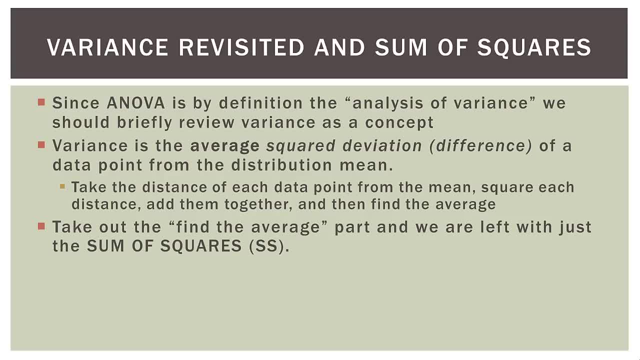 If we stop there, That is the sum of squares. So the sum of squares is variance without finding the average of the sum of the squared deviations. So it's the variance without that last step. And that's because sum of squares is a foundational component of ANOVA. 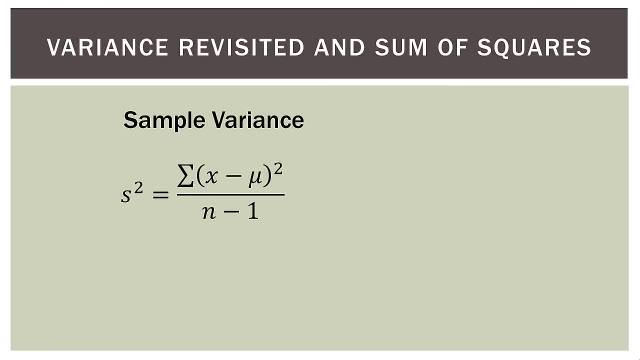 So remember the formula for the sample variance. That's what we just talked about. It is the sum of the squared deviations divided by the sample size minus one in the sample case. So on the top we have the squared differences. So remember x is the data point. 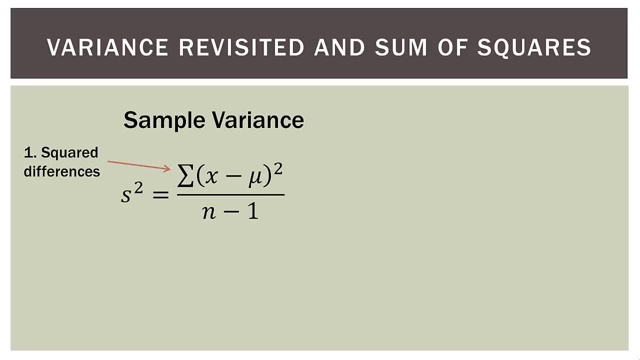 minus mu, which is the mean. We take that difference and we square it, We sum all those up And then, in this case, we divide by n minus one. So on the bottom we are doing the averaging of the squared differences. 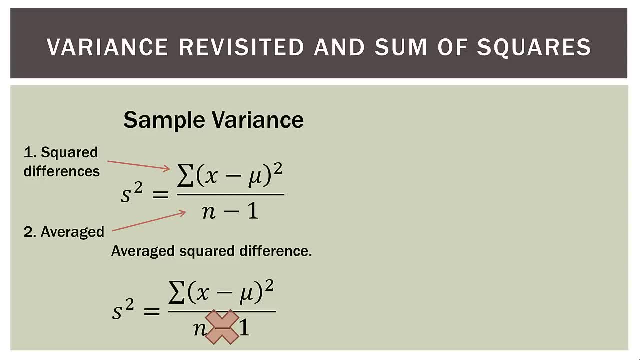 Well, what if we take away the n minus one part? Well, we are just left with the sum of the squared differences. Well, we are just left with the sum of the squared differences. So, each data point minus the mean Square it. 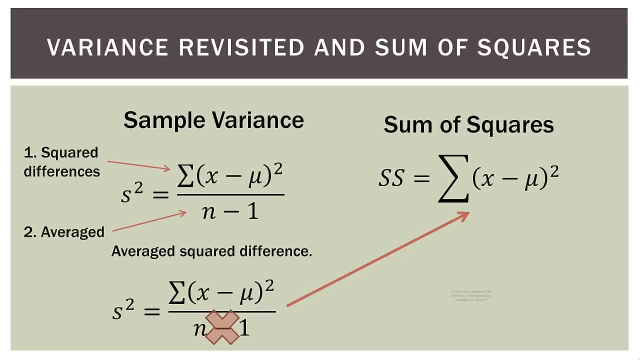 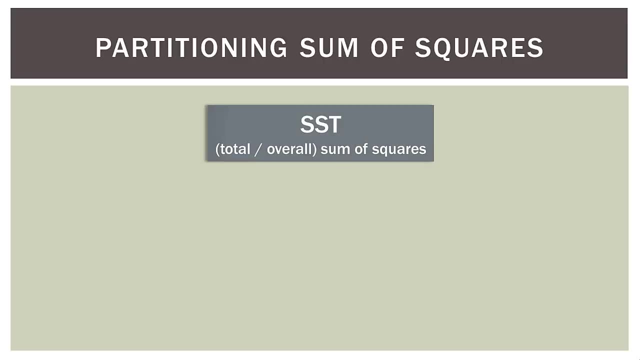 Do that for all the data points, Add them up And that is the sum of squares. So we have the sum of squares of the difference between the dependent variable and its mean. That's all. the sum of squares is Now, when we talk about sum of squares in the ANOVA context. 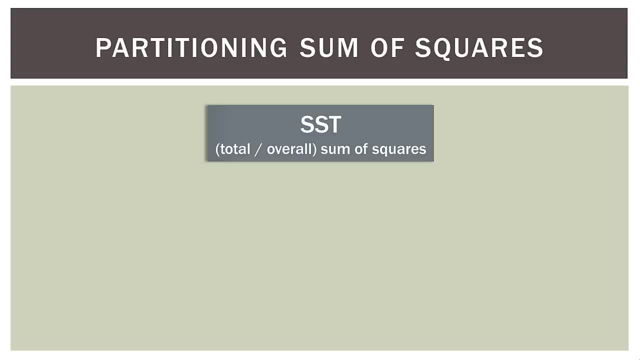 what we do is we say this overall sum of squares is partitioned or split into two parts. So we call the total sum of squares SST, That's sum of squares total. Now that's made up of two components. The first component is the SSC. 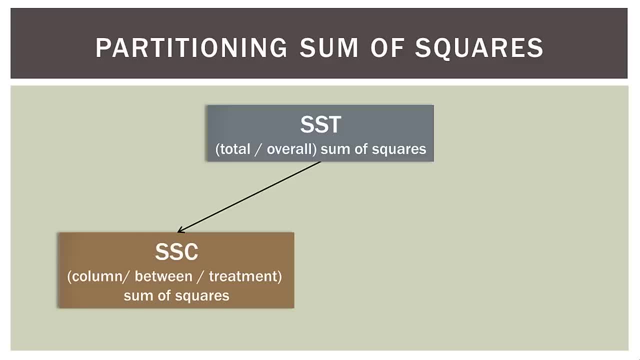 That is the sum of squares of the columns. So the columns, the between variance, the treatment sum of squares. That's what we are talking about And again, this will make sense more in a minute when we look at the actual problem. 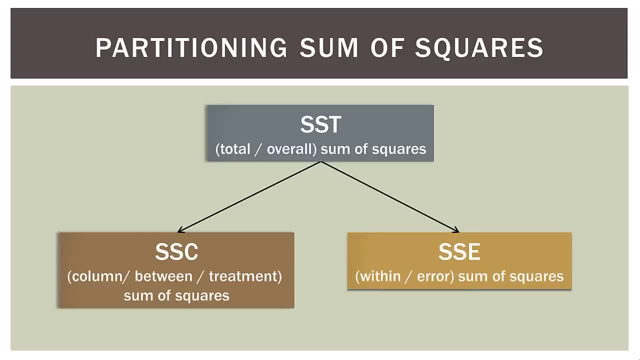 And again, this will make sense more in a minute when we look at the actual problem. Now the other component is the SSE, which is the sum of squares error. So this is the within or the error sum of squares. So the overall or total sum of squares in the one-way ANOVA. 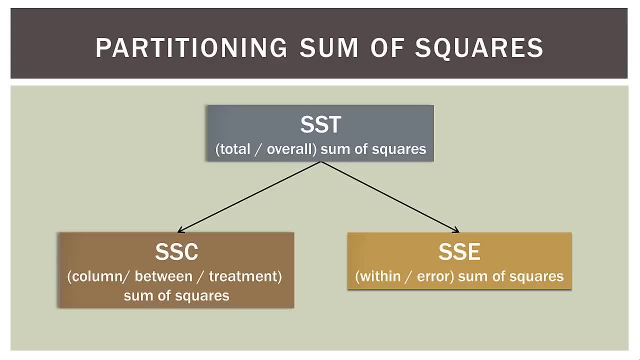 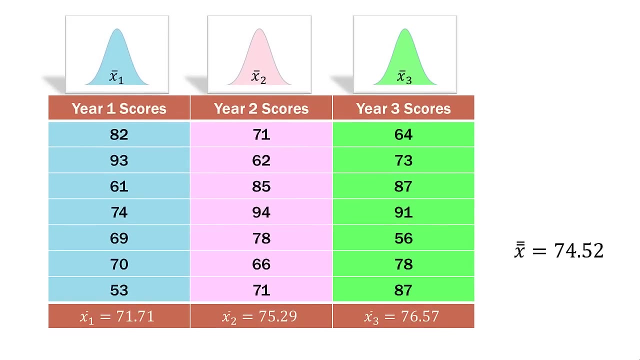 is actually a combination of two things: The sum of squares of the columns, sort of between the columns, and the sum of squares of the error, which is actually the sum of squares within each column. So let's look at each one of these types of sum of squares. 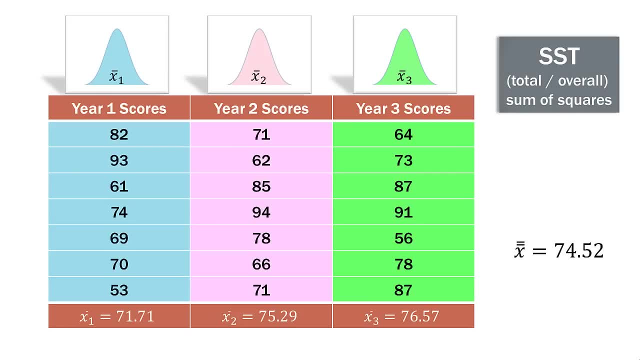 using our actual data. So we'll start with SST, or the sum of squares total. So what we do is we find the difference between each data point, so all 21 data points and the overall mean over here on the right-hand side of 74.52.. 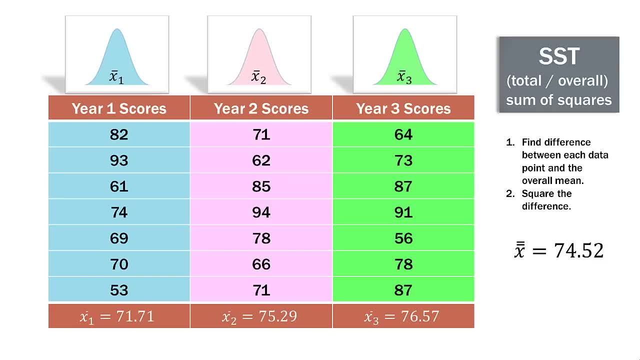 We would then square that difference and then add all of those up, So we would have 21 squared differences. So here I only circled five, but we would do this with all 21. So it's the difference between each data point. 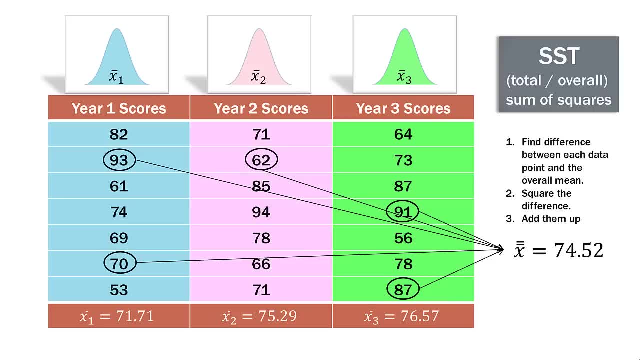 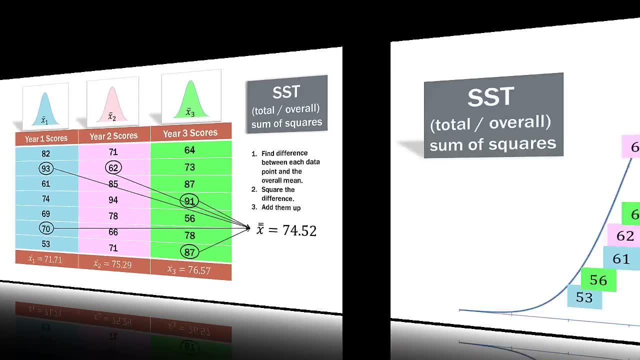 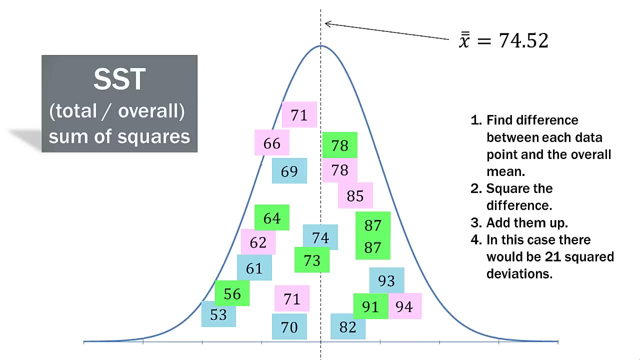 and the overall mean. square it and then add them all up. That is the sum of squares total. So if we look at this in the actual distribution, we have all 21 of our data points put together And then we have the overall mean of 74.52. 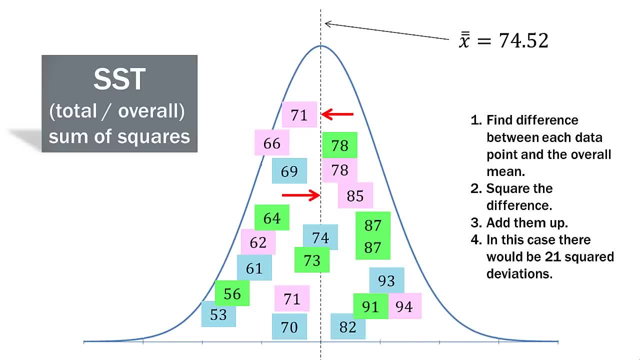 in the distribution there. So what we're doing is we are finding the distance of each data point to the overall mean, And then, of course, we square it, So we would have 21 squared deviations. Now, here's the thing. 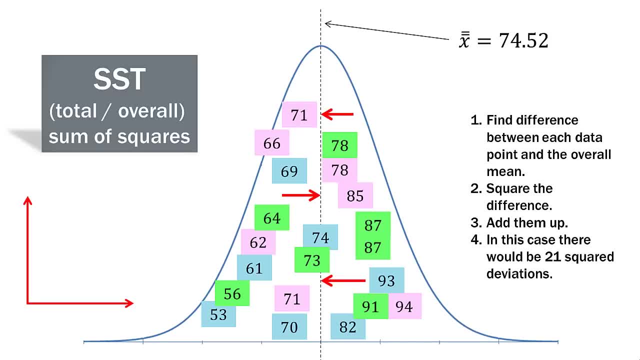 When we take a distance and we square it, guess what we get? We literally get a square. So when we say sum of squares, we actually mean that literally. So we take every distance, from the point to the mean we square it. 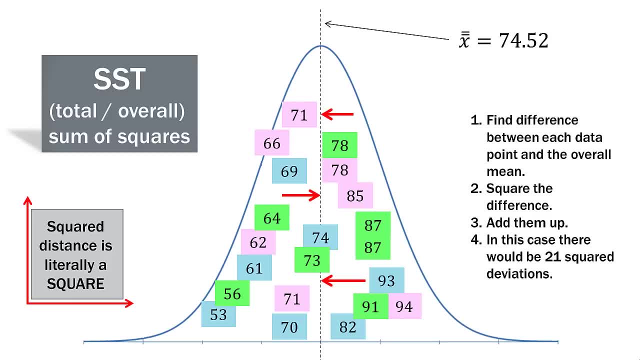 So we would have 21 individual squared distances on this graph if we actually did it, And then we sum up the area of all those squares. Now I only mention that because it's gonna become an important part later on when we talk about regression. 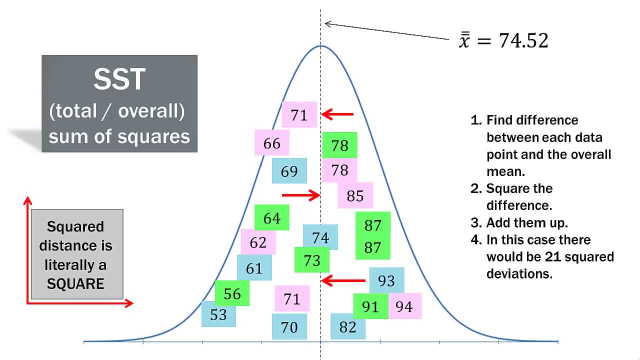 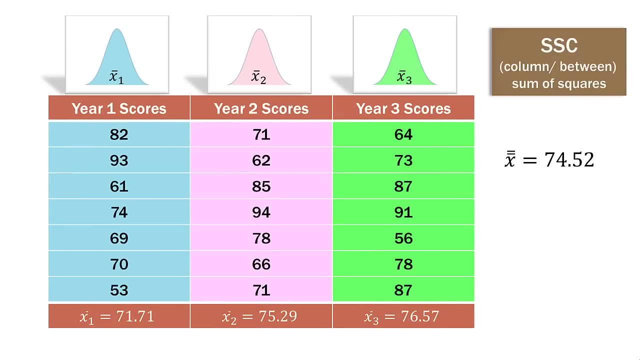 because sum of squares is a very important part of regression as well. So sum of squares is literally square distances when added together, or the bunch of squares added up. Now let's look at SSC, which is the sum of squares of the columns. 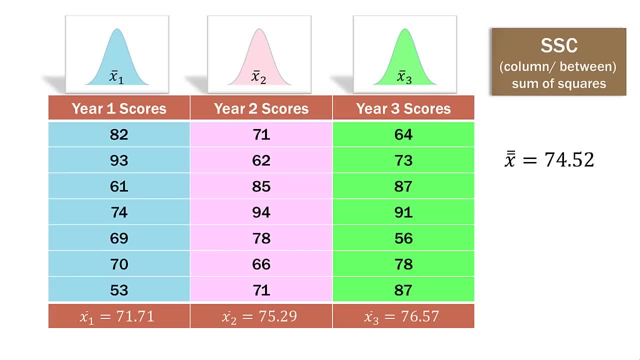 So this is the column or the between sum of squares. So in this case we find the difference between each group mean and the overall mean, square those deviations and add them up. So the SSC is the difference between the individual column means. 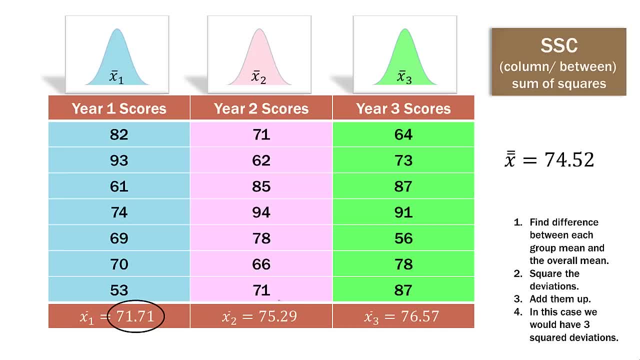 and the overall mean. So in this case we'll have three. So each individual column mean and the overall mean. So remember the SST, or the sum of squares total, was the relationship between each individual data point and the overall mean. 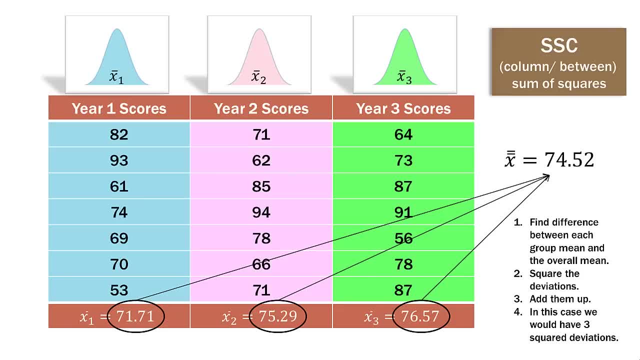 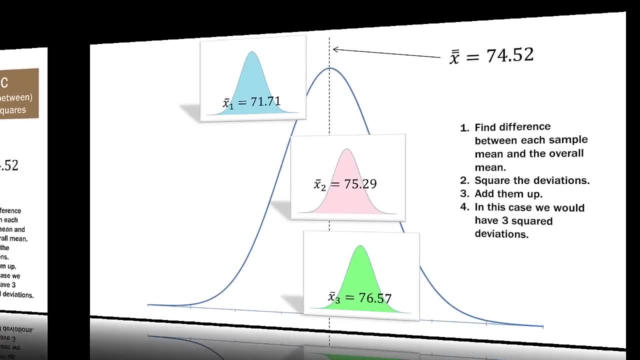 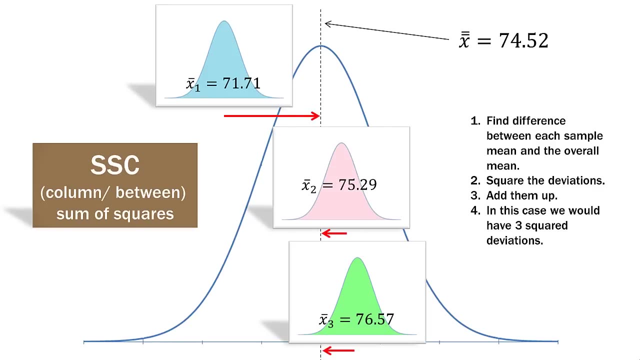 Well, the SSC, or the sum of squared columns, is the relationship between each column mean and the overall mean. So that would look like this: So the SSC is the distance from each mean to the overall mean. So you can see that there in the red. 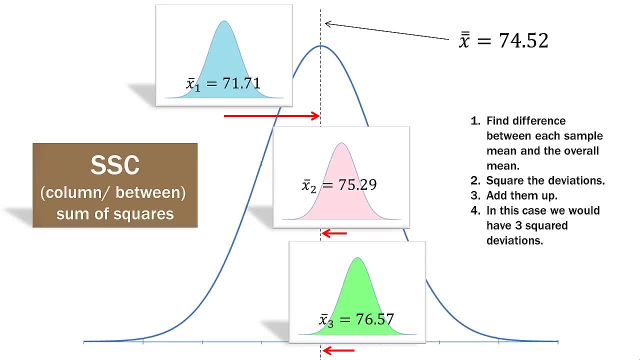 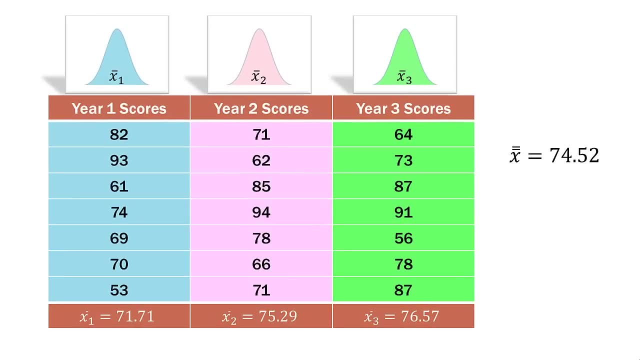 And again, in this case we would literally have squares. So the squared distance or the squared deviation, add them all up Now. the third type is the SSE, That is, the sum of squared error or the within sum of squares. 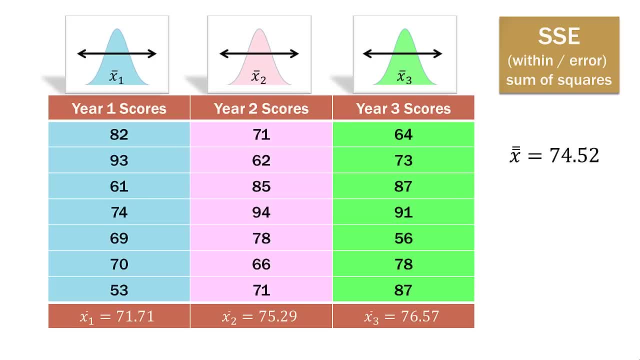 So this is actually about the individual distribution around each column mean. We're not dealing with the overall mean in this case. So we would find the difference between each data point and its own column mean, Square each deviation and then add them up. 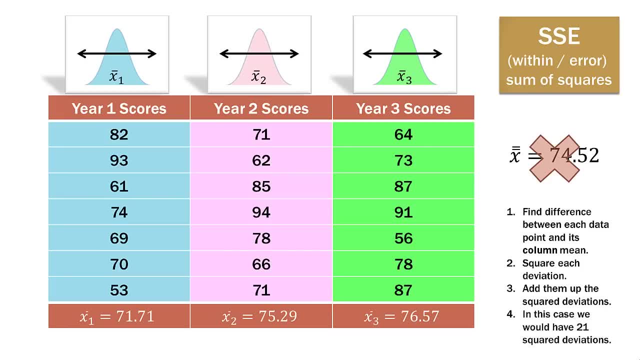 So, for example, we would have 21 squared deviations in this case, Because we would take each column score and then find the relationship between the overall column mean. So the difference between each data point and its corresponding column mean, Find the difference. 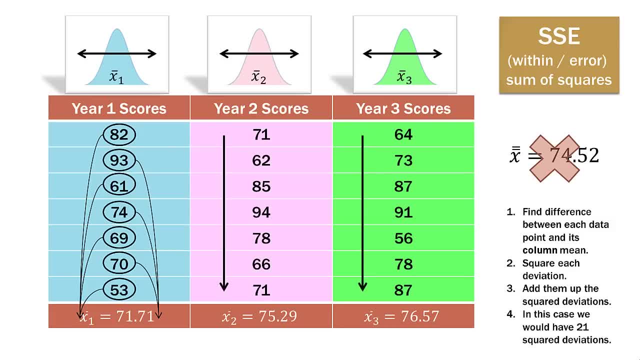 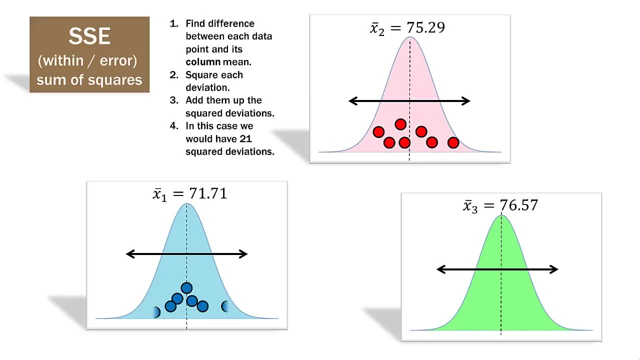 square, it add them up, And then we would do the same thing for each column. That is SSE, or the sum of squares within. So what we're looking at here is the distribution within each column, So where each data point falls. 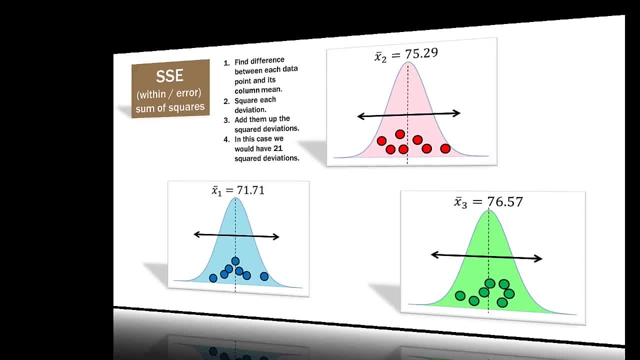 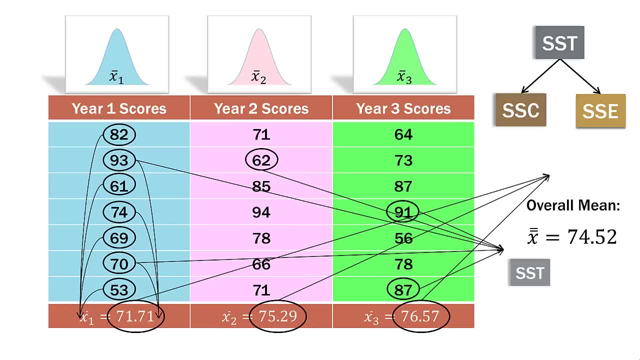 within each column. So this is what these three types of sum of squares look like when we put them all together. So in the first case we have SST. Remember that is each individual score. so all 21 scores as they relate to the overall mean. 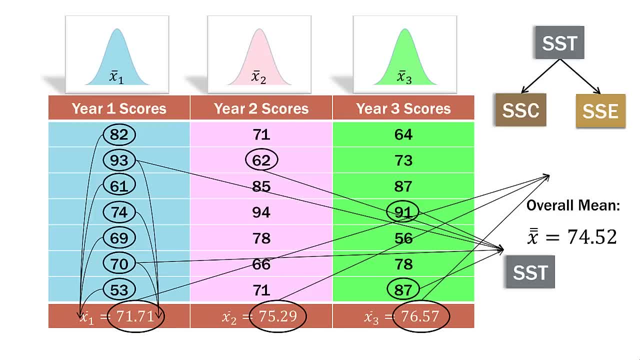 So we find the difference between each score, the overall mean, square it. add them up. The SSC is the relationship between each column mean there at the bottom and the overall mean. So we find the differences, square them. 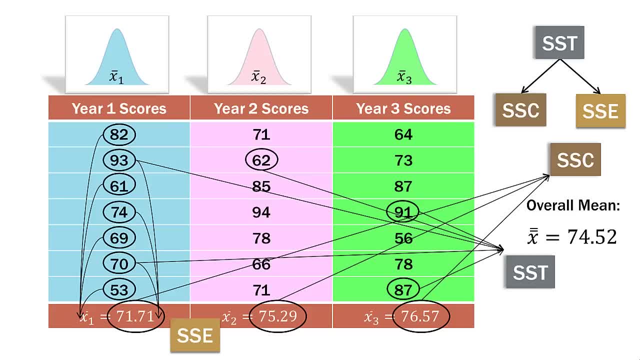 add them up. Then the SSE is the relationship between each individual score and its own column mean at the bottom. So we find the difference between those two square. it add them all up So you can see the three different ways. 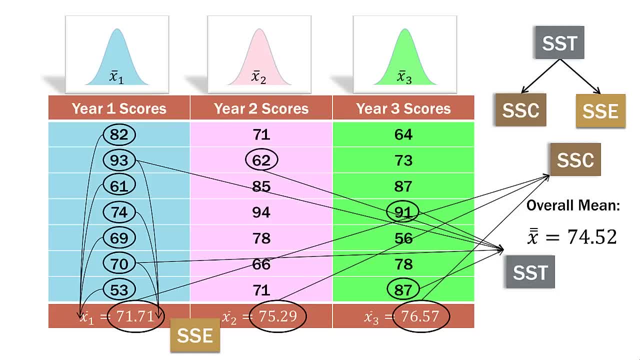 we're looking at the sum of squares And the cool thing is is that the SSC- the sum of squares columns plus the SSE sum of square error, adds up to the SST or the total sum of squares. So you can see all the ways. 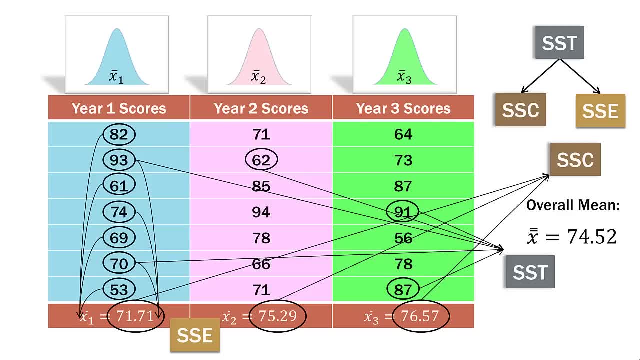 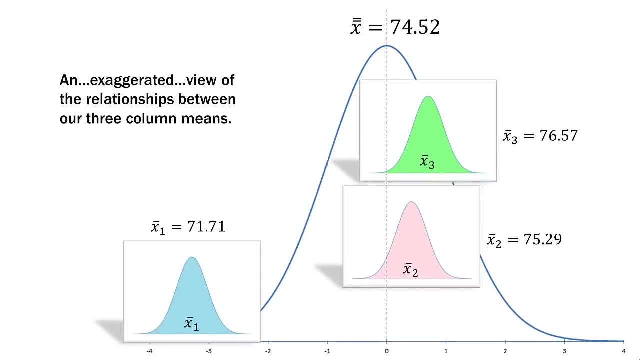 the data is sort of parsed when we do the one-way ANOVA. So this is an exaggerated view of the relationship between our three column means. So you can see that group one, or the first year students, had a mean of 71.71.. 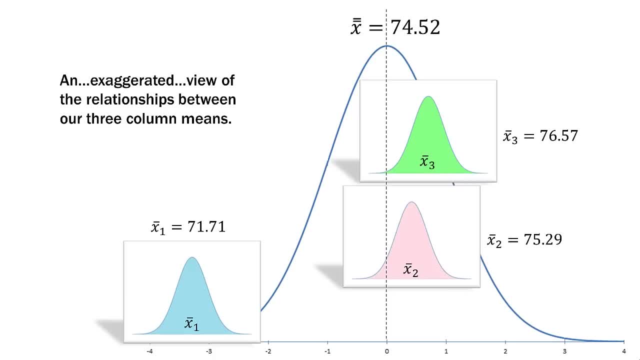 The year two students had a mean of 75.29, there in the pink, And the year three students had a mean of 76.57, there in the green, And I've kind of exaggerated the distance of group one So you can see that each distribution. 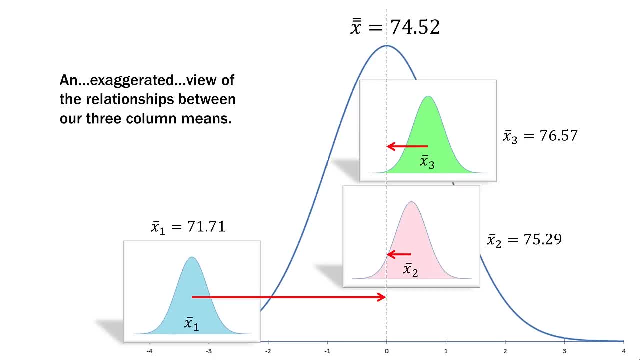 or each column has its own distance to the overall mean. So what we're trying to figure out here is: is the first year student distribution, those scores kind of an outlier or sort of an oddball distribution? That's what we're checking for. 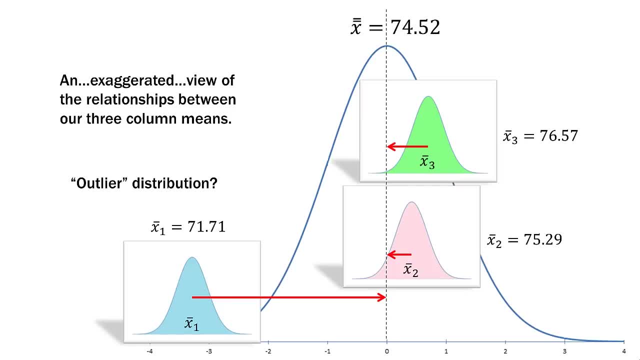 when we're doing the one-way ANOVA. Now, remember, in the previous video I talked about why we cannot do- we cannot do- three pairwise t-tests So we could compare group year one to year two, year one to year three. 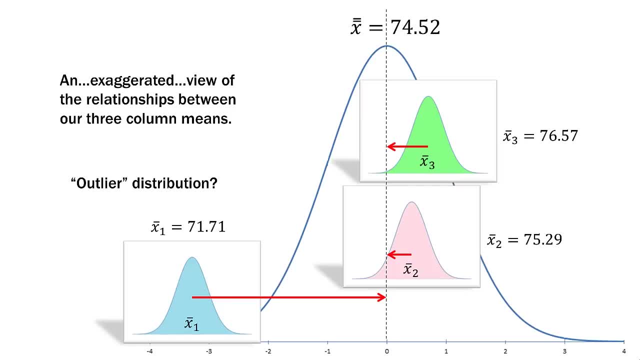 and year three to year two. That would be three individual t-tests. We cannot do it that way because the error, the type one error, compounds each time we do that And we end up with a type one error rate of over 14%.